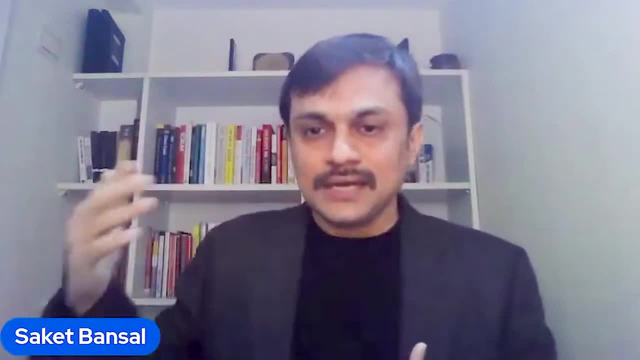 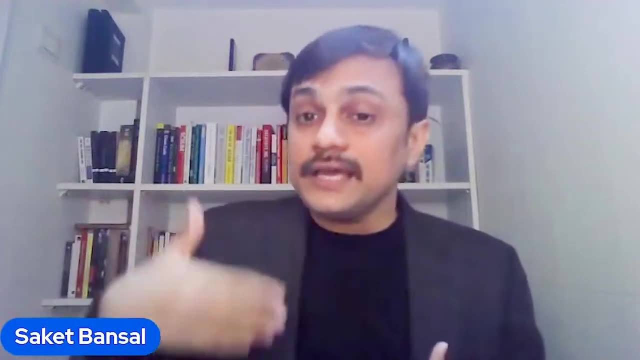 project life cycle, be it productive, be it agile, be it hybrid. Estimation means you estimate all the time, multiple times at least. in the productive way world, we say each phase end, you should be re-estimating. In an adaptive world we can say: 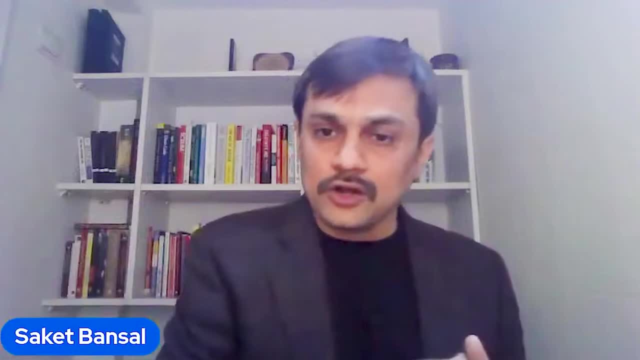 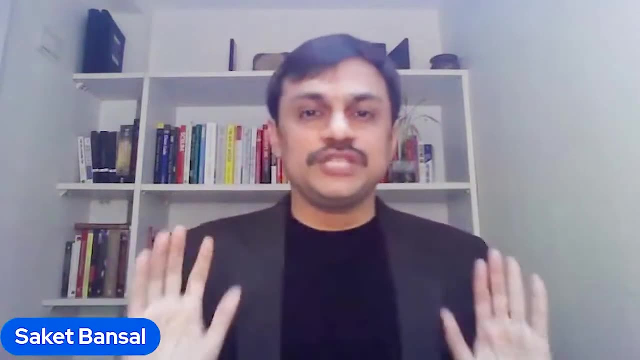 the backlog. refinement is a continuous estimation of the product backlog and you estimate to find out what can I do in a given iteration. So with this context we should approach the estimation Now. there could be an organizational challenges and interpretation challenges, but this is how. 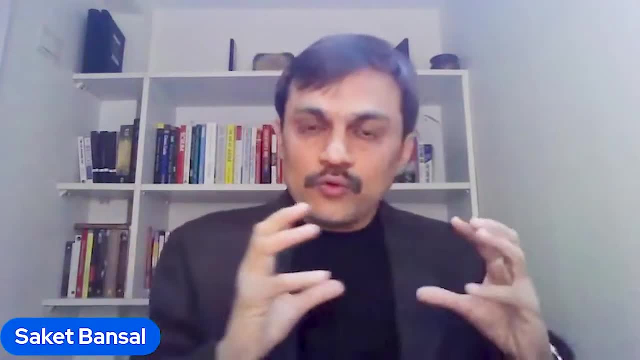 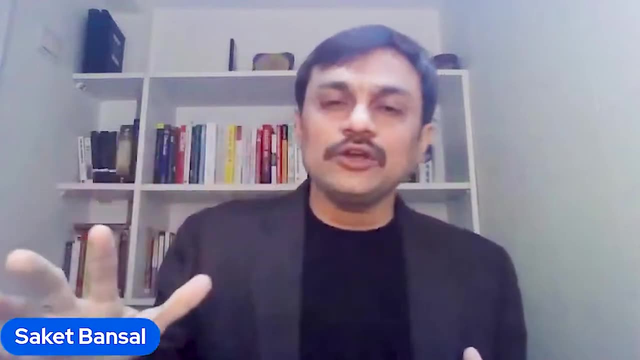 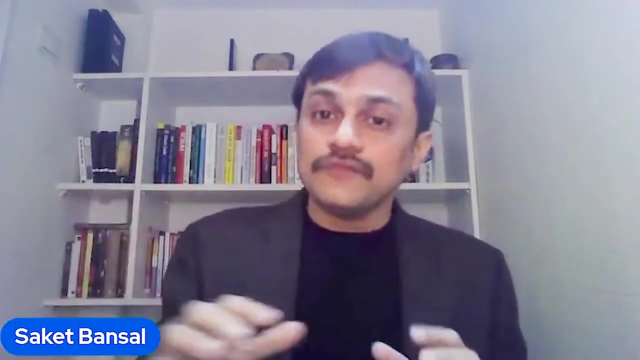 the overall approach of estimation is designed. Now, when you are estimating at a big level, say epic level, project initiative level, you might make some understanding of what all will go into it, say a set of features or some references And, based on the judgment of 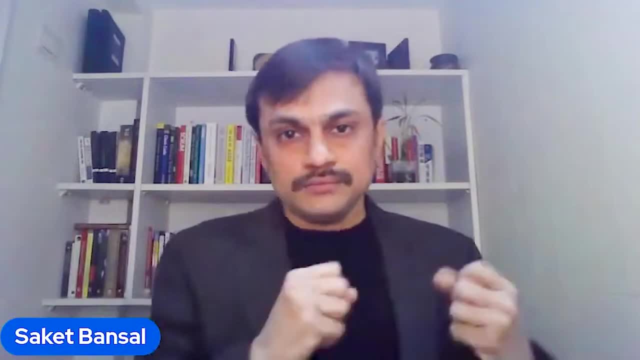 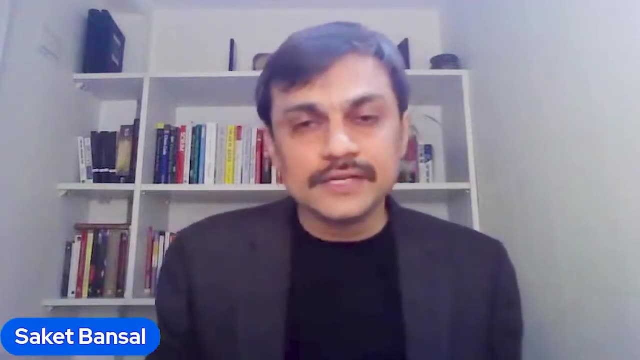 individuals who are available at that point in time, because a lot of people who will come and develop it may not be even identified at that point in time. So whoever is available, they will make their judgment based on whatever historical data they have. So they may have a set of 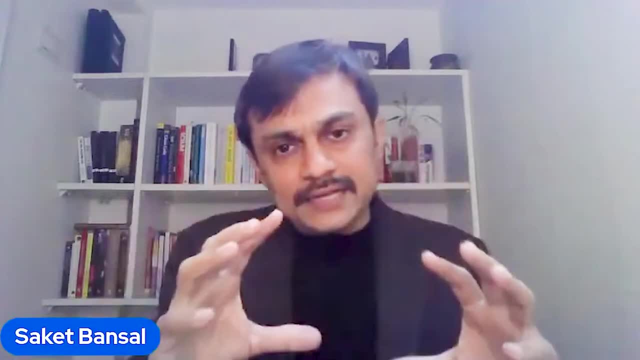 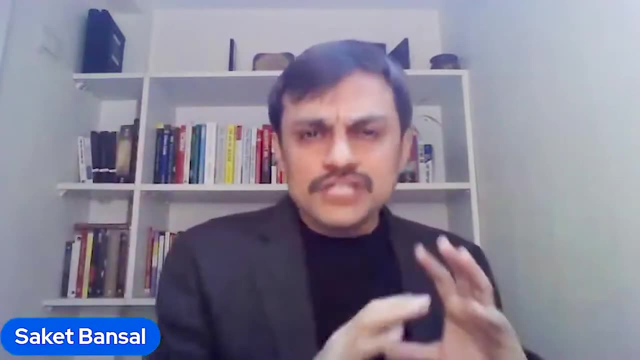 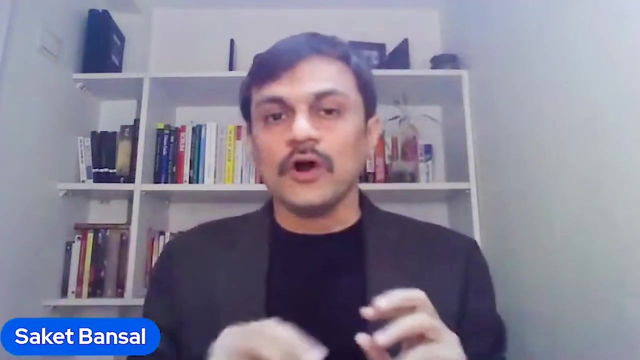 different large initiative to come. What they may divide that initiative epic into features and they compare those features into the existing historical data. But depending upon which framework you are using, you may use terminologies, But idea here is that is done based on historical data comparison. You can call it. 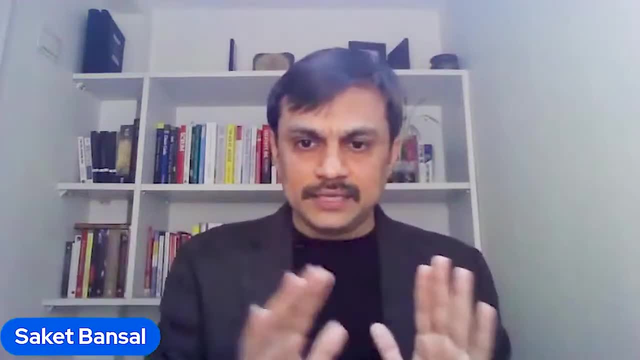 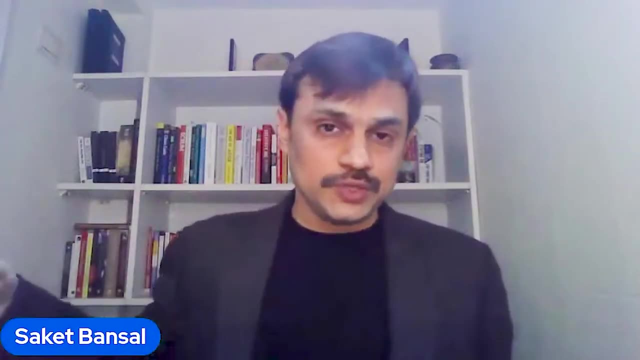 analogous estimate and you compare with something, You compare there, and then you come up with it And you also put it that, okay, there could be a variability attached to it. Now, how much variability? It also depends upon how well you are able to compare it with the existing historical data. 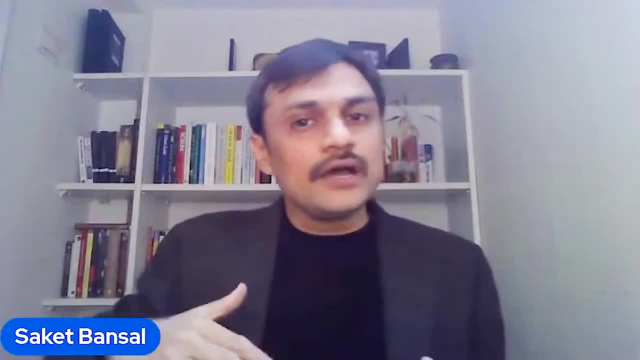 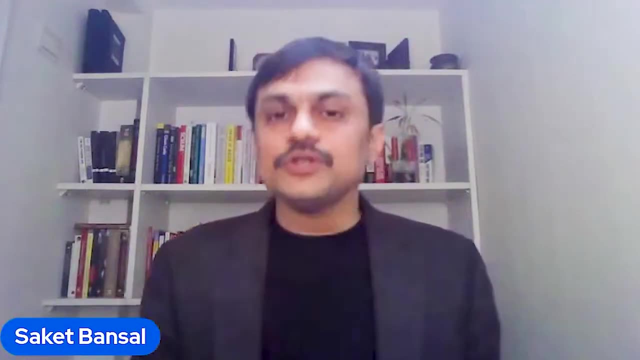 Well, that particular initiative is understood. If you are getting into a very unknown territory, your error could be more than 500%. If you are getting into a known territory where your customer persona is known, your platform is known and you just need to get into that particular. 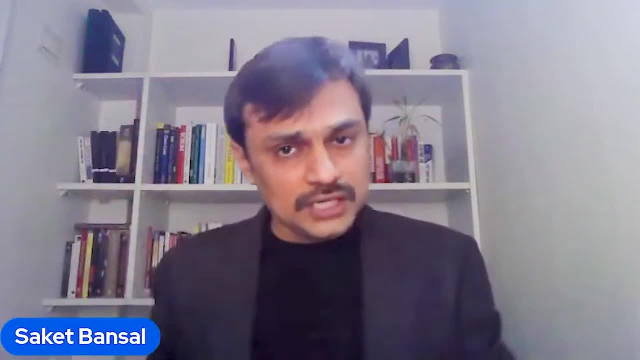 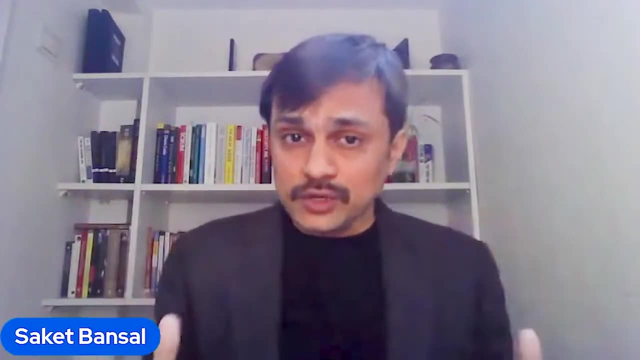 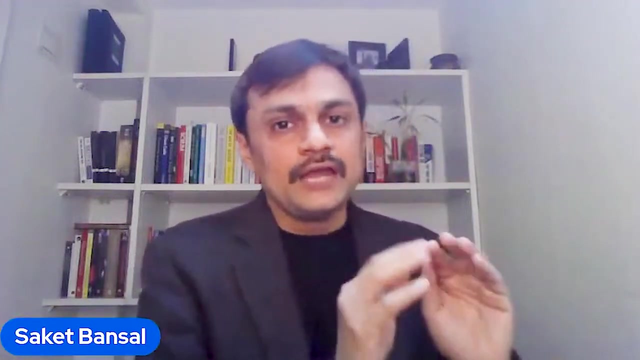 space. your estimation error at a large initiative to real detailed estimate later on comes in or real one comes in, maybe 50%. So it depends, And, as a stakeholder, what we need to do is make our best guess, Whatever information is available at that point in time and focusing on the utility of it. Now, if we